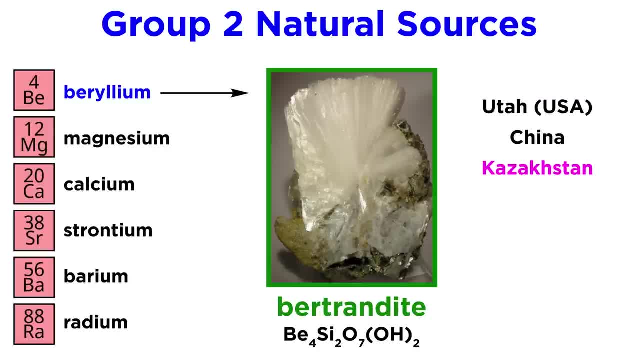 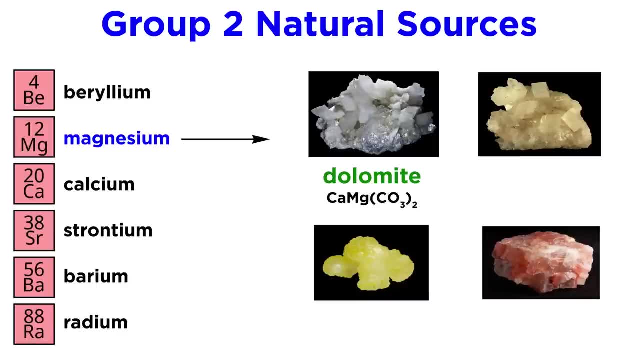 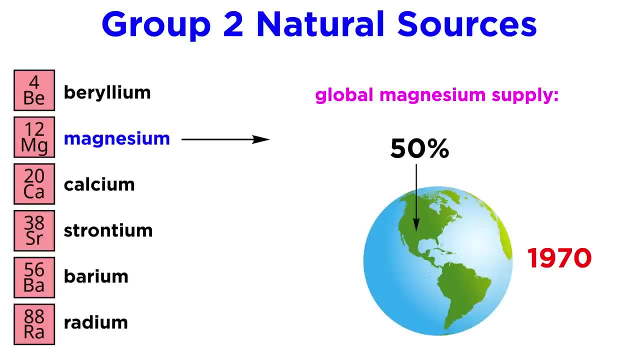 the United States, but also in China and Kazakhstan. It is rare and expensive. Magnesium is found in a variety of ores such as dolomite, magnesite, brucite, carnelite and others. Only a few decades ago, the United States produced around half of the. 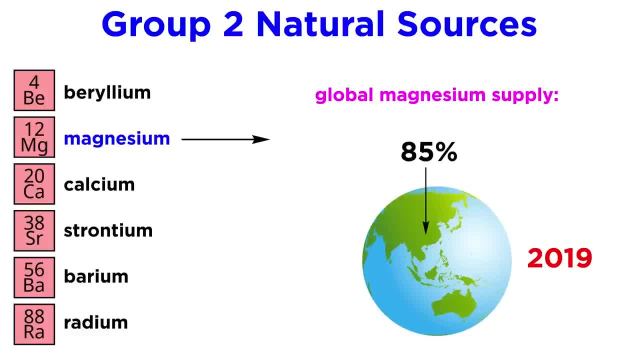 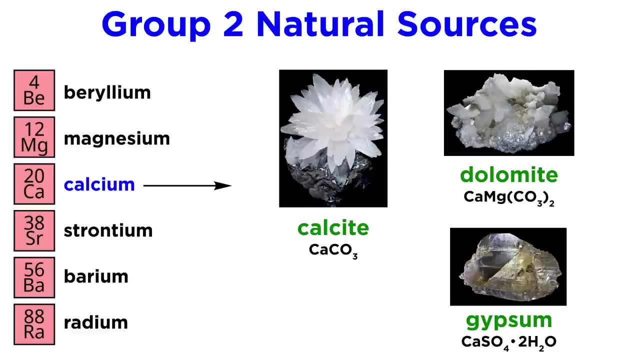 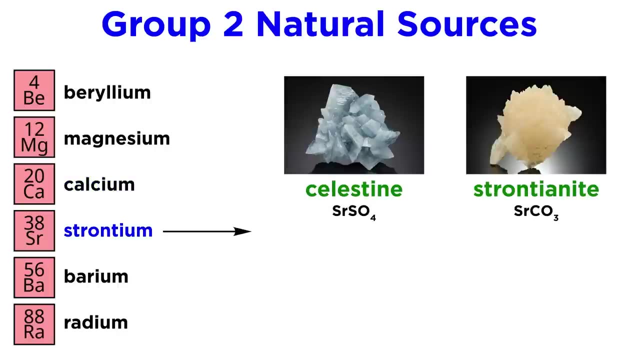 magnesium in the world, while, as of 2019, China has produced about 85%. Calcium is found in the ores, calcite, dolomite and gypsum. These are widely abundant, primarily in Spain, Iran and the United States. Strontium is found in celestine and strontionite. 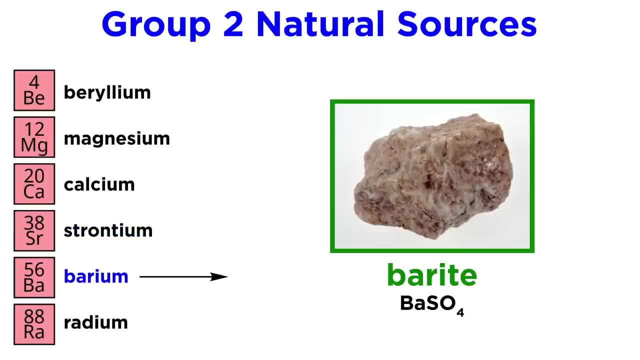 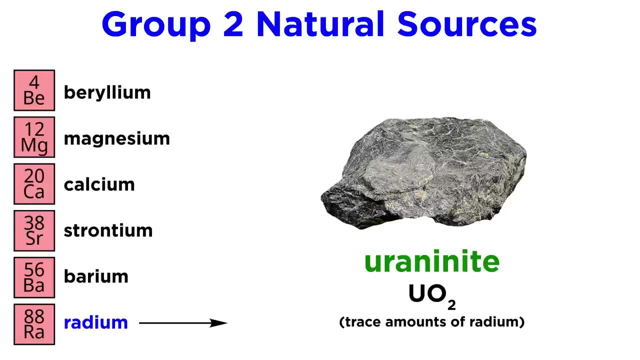 again with China and Kazakhstan. In addition, beryllium is found in a variety of ores such as magnum cadmium and cadmium acting as the primary producer. Beryllium is found in beryte. And finally, radium is found in trace amounts in uranium ores. 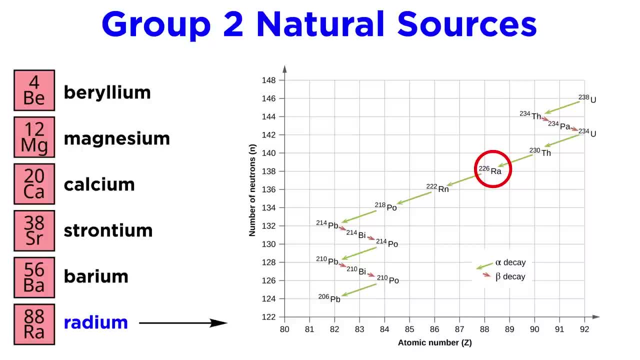 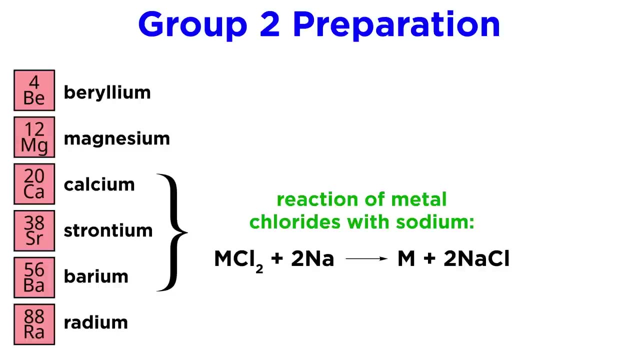 like uraninite. This is because it is part of the decay chain for radioactive uranium nuclides, and one ton of uraninite will produce 150 milligrams of radium. Now, natural sources aside, how are these elements prepared? Calcium, strontium and beryllium are produced by the formation of a mixture of radioactivity and radioactivity. The radioactivity, which is known as radioactivity, is a good source of radioactivity. for radioactivity, However, beryllium is found in the form of radioactivity, which is the main source of radioactivity. 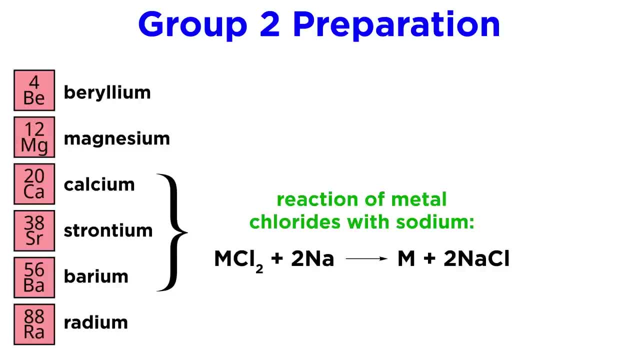 reacting metal chlorides with sodium, yielding pure metal and sodium chloride. Magnesium is produced by electrolysis of magnesium chloride, calcium chloride and sodium chloride. Another method involves reacting magnesium oxide with coke carbon to produce magnesium metal and carbon monoxide. Beryllium is produced by reacting beryllium chloride with magnesium. 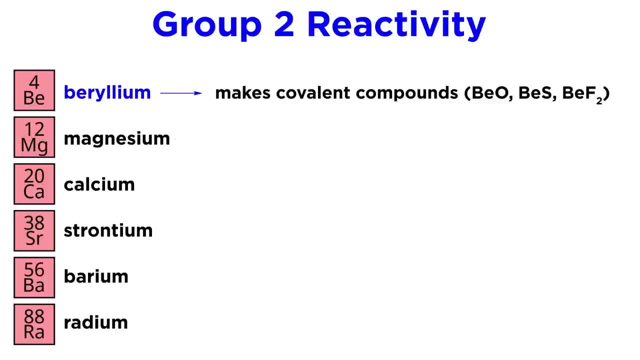 or calcium. In terms of reactivity, beryllium makes mainly covalent compounds like beryllium oxide, beryllium sulfide and beryllium fluoride. It can also bond covalently with carbon. Magnesium. 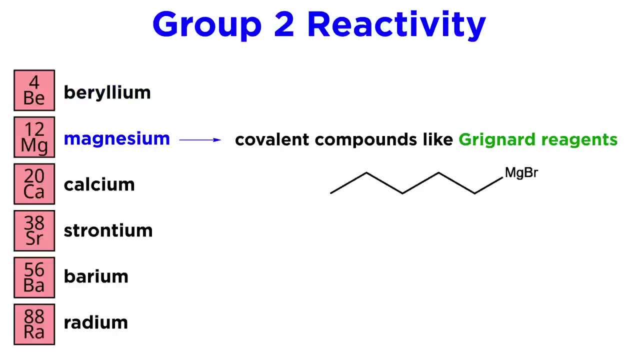 has some tendency towards covalency, especially with carbon, such as with the Grignard reagents we should be familiar with, but it can also make ionic compounds like magnesium oxide and magnesium hydroxide. The other members of the group make lattice hydrates with halide ions with lower stability. 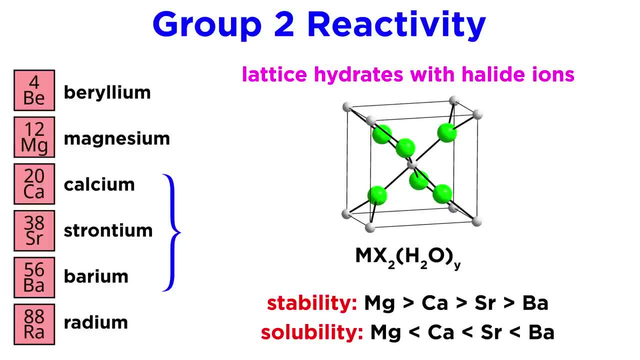 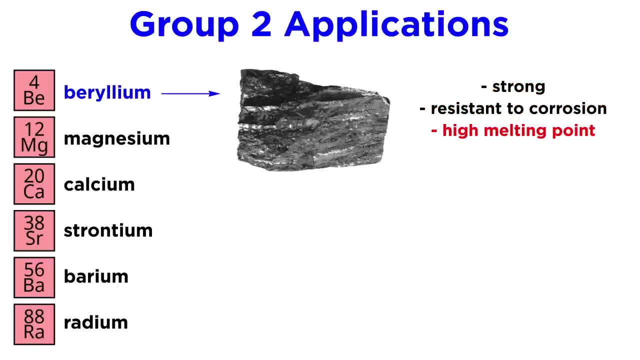 and greater solubility as the metal cation gets larger. Looking at applications, beryllium is strong, resistant to corrosion and melts at high temperatures, though it is somewhat toxic. Nevertheless, these properties make it quite valuable and with 60% of the world's. 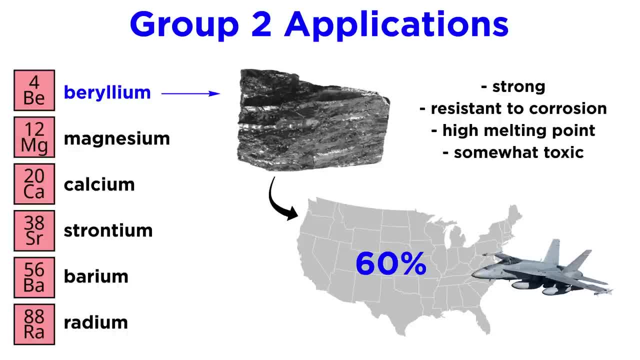 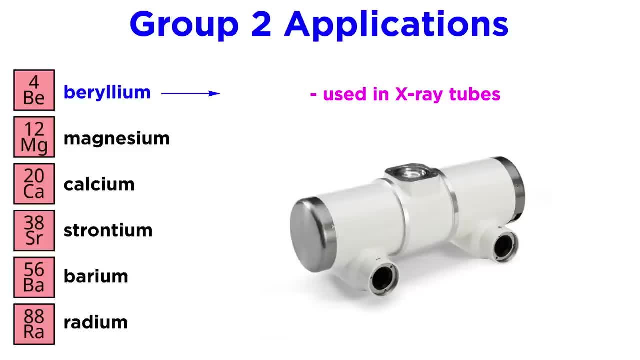 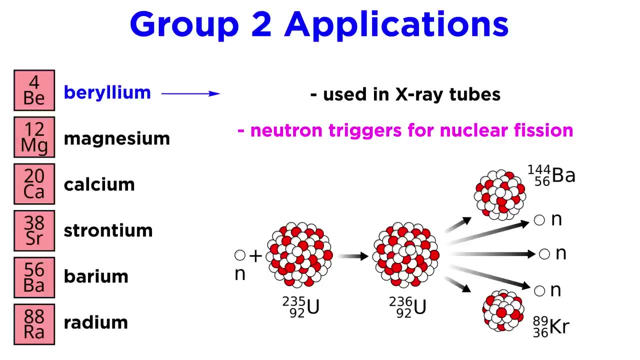 supply. in the United States, it is used largely for military applications. Beryllium is also used in X-ray tubes, as it is transparent to X-rays and also strong enough to keep a perfect vacuum. Other applications include neutron triggers for nuclear fission beryllium. 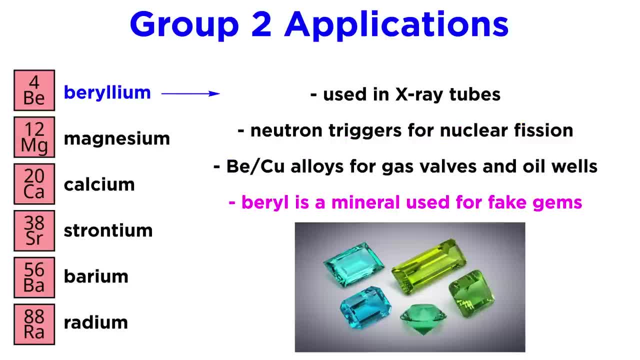 copper alloys for gas valves and oil wells and a mineral called beryl which can take on either an aquamarine or emerald color and is used to make fake gems. Magnesium is moderately priced, strong and light and quite flammable. Magnesium is both oil and 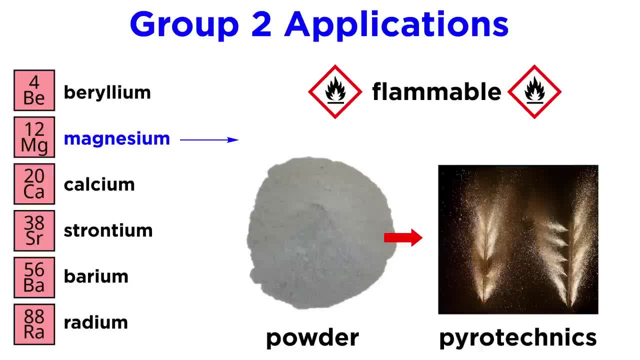 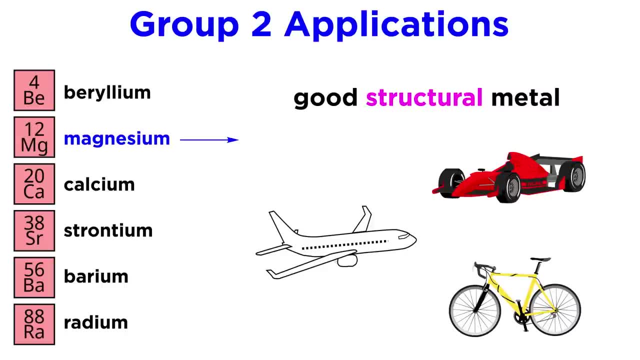 copper, and it can be used to make natural chemicals like potassium, zinc and iron, whether in ribbon or powder form, with the latter form being used in flash powders for pyrotechnics. It is the first industrially useful structural metal in the periodic table. 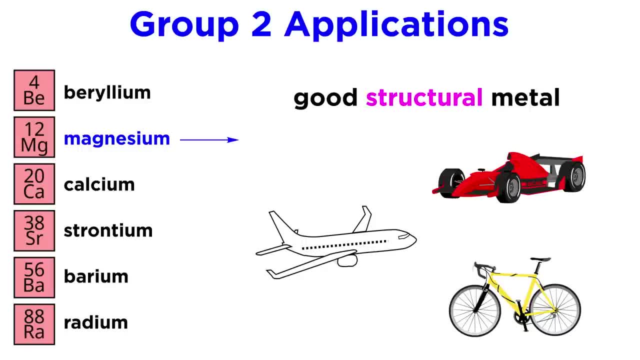 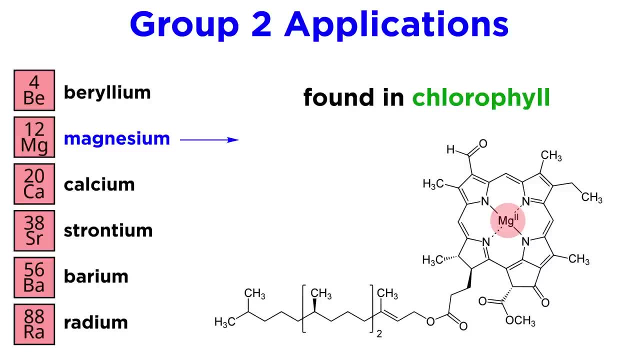 used in race cars, airplanes and bicycles. Magnesium also has a very important role in nature, sitting in the center of the porphyrin ring in chlorophyll, the pigment molecule which initiates photosynthesis, a process which all life on earth depends on either directly or indirectly. 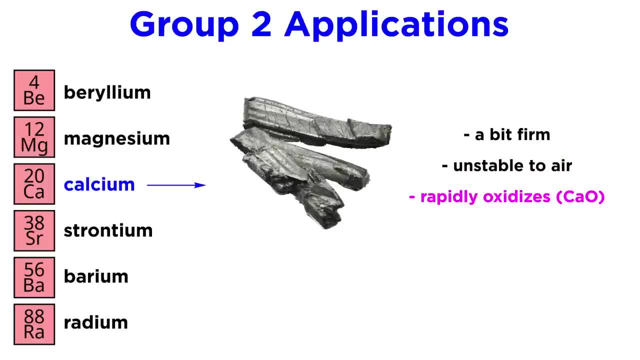 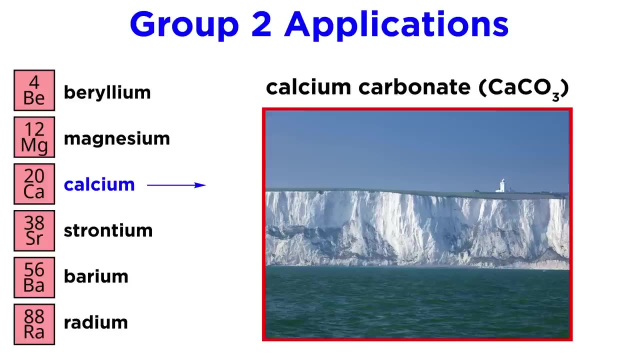 Calcium is a bit firmer and is unstable to air, rapidly oxidizing to form calcium oxide. Calcium can react with water to form calcium oxide and hydrogen gas. Calcium carbonate is a very important compound which we know of as chalk, such as what is found on the famous White Cliffs of Dover, as well as in seashells and corals. 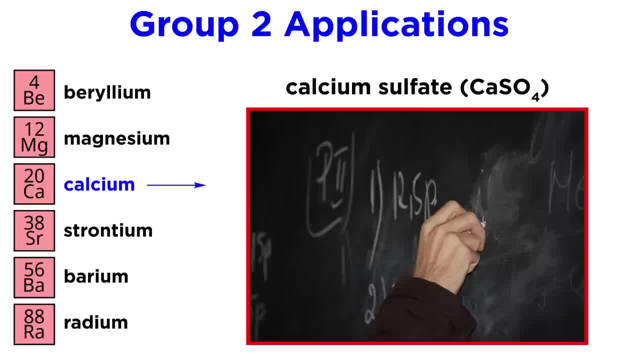 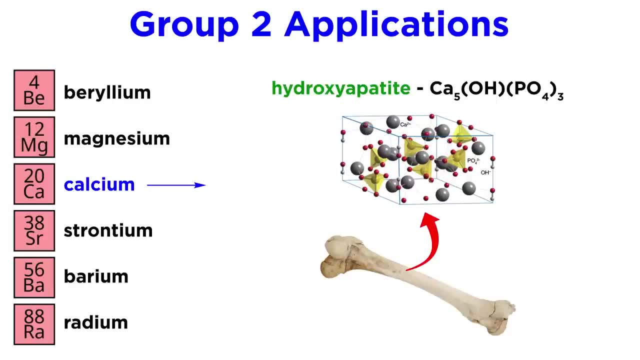 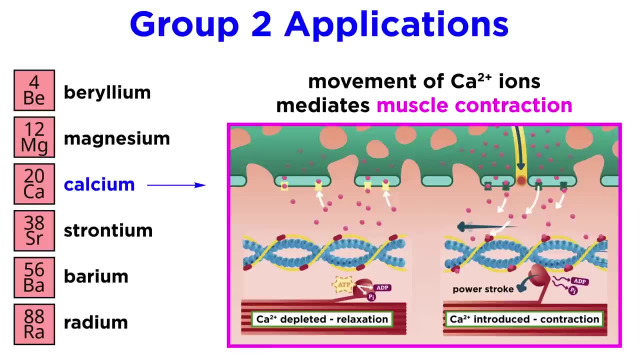 Blackboard chalk, rather, is calcium sulfate. Calcium is crucial to most animal life, being that bones contain a rigid hydroxyapatite foam, which is a form of hydrated calcium phosphate. Additionally, the movement of calcium ions across the membranes of nerves and muscle cells mediates muscle contraction, so we literally would not be. 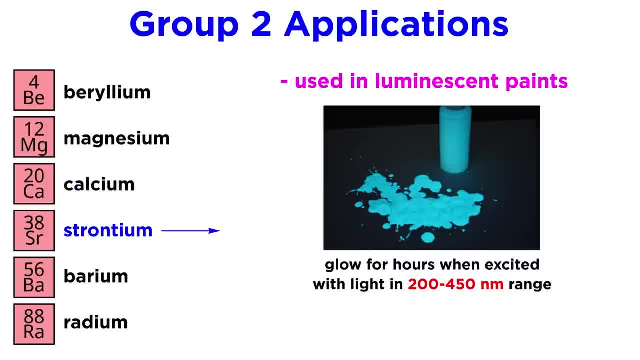 able to move at all without this important element. Strontium is used to move from the stressor to the muscle cells and is used to plant herbs like green onions and other animals' food. Calcium is also used to produce fish fish's food. 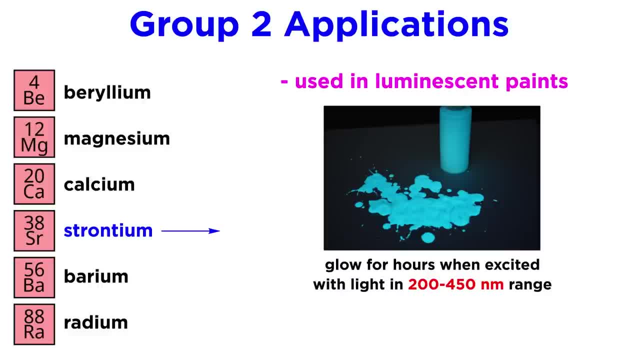 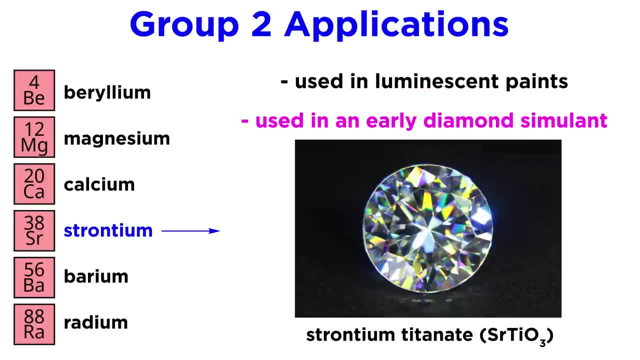 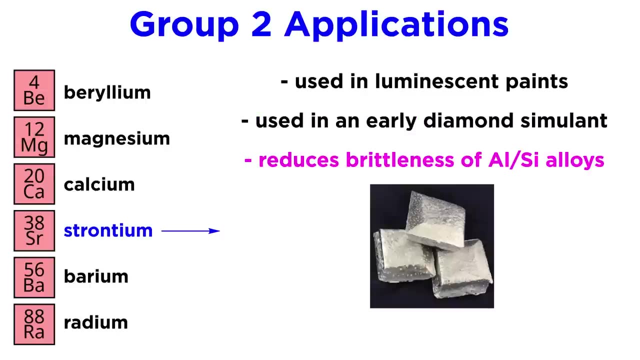 in luminescent paints which glow for hours after excited with light in the 200 to 450 nanometer range. It was also used in an early diamond simulant prior to the popularization of cubic zirconium. Strontium is used to reduce the brittleness of aluminum-silicon casting alloys. 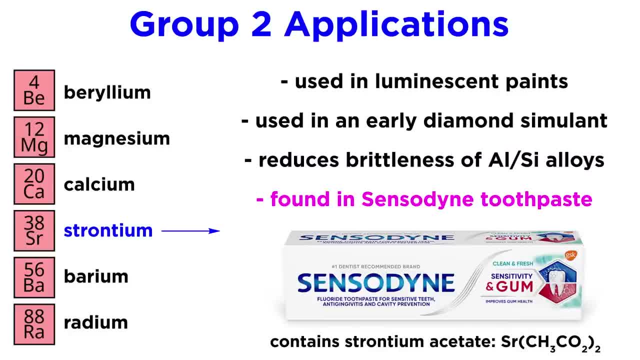 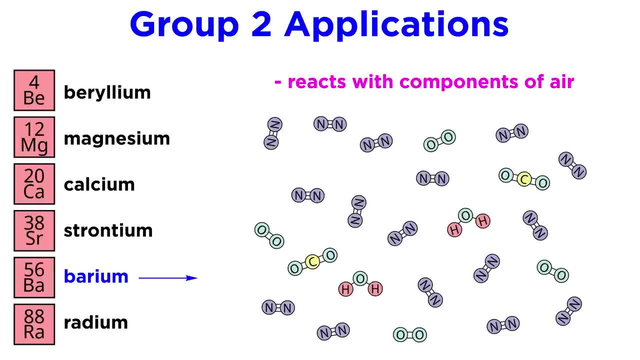 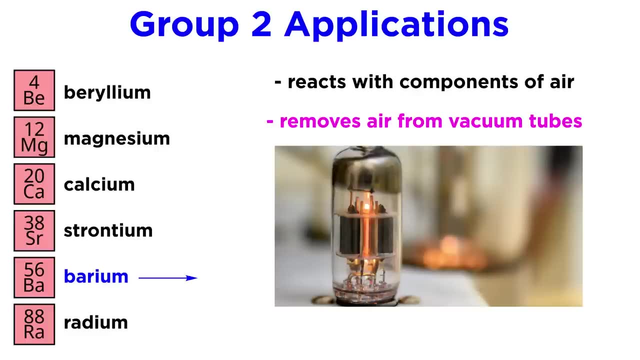 and it is found in the active ingredient in sensodyne toothpaste. Barium reacts with everything in the air, like oxygen, nitrogen, carbon dioxide and water, thereby allowing for the removal of air from a particular environment, like vacuum tubes within electronics Barium. 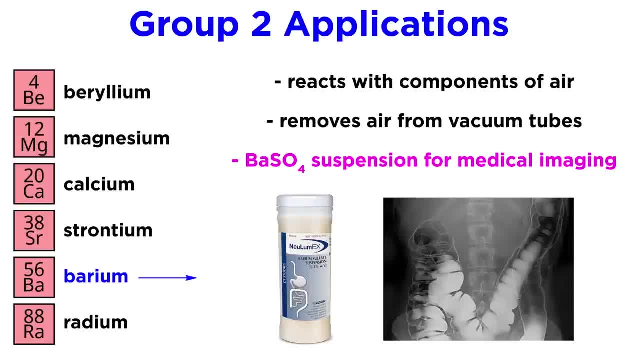 sulfate has application with medical imaging, where patients drink a suspension of the substance, and this allows for X-ray imaging of the digestive system, due to this material's ability to absorb X-rays very well. Barium is also found within certain superconductors. 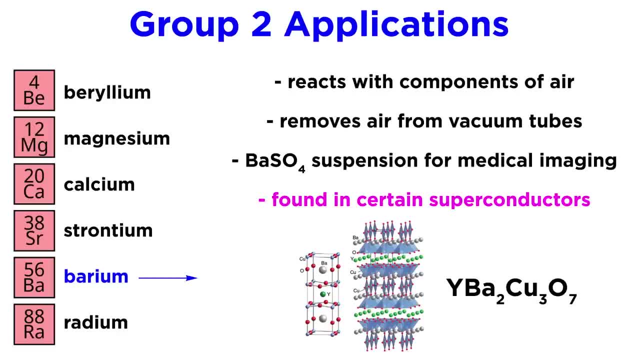 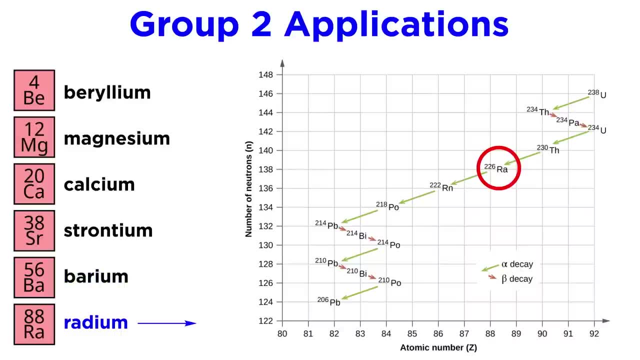 like oxygen, nitrogen, carbon dioxide and water, thereby allowing for the removal of air from a particular environment like this one, which superconducts at liquid nitrogen temperatures, thereby not requiring the greater difficulty of utilizing liquid helium And radium is a 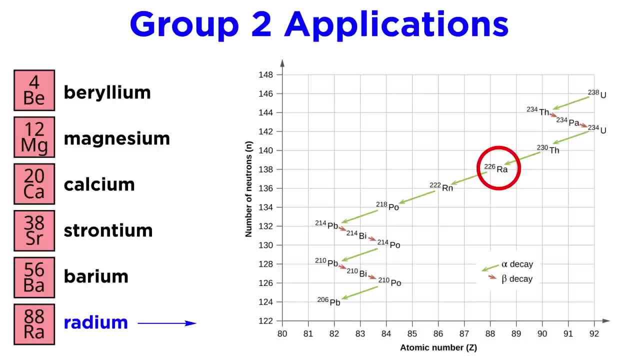 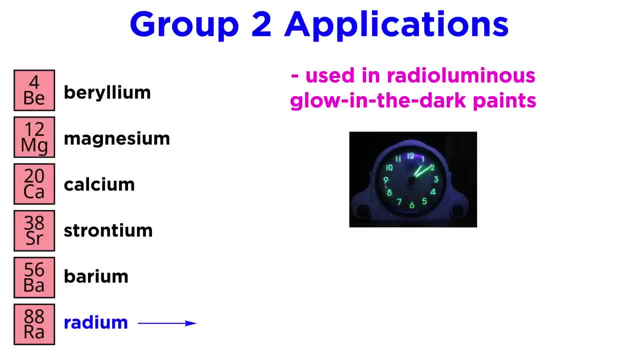 naturally radioactive element which forms from the decay of uranium. All isotopes of radium are radioactive. This element was used in radioluminous glow-in-the-dark paints in the early 1900s, where a small amount of radium was mixed with luminescent zinc sulfide. The radiation from 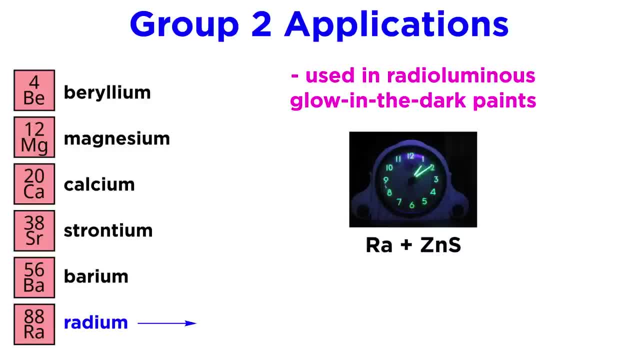 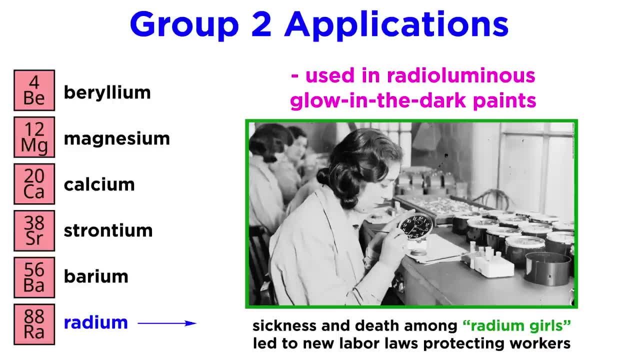 the radium was absorbed by the zinc sulfide, which produced a glowing effect, and this was useful for various purposes in World War I. It slowly became understood that this was not a safe material to use as so-called radium. girls were in the habit of sharpening paintbrushes by licking them. 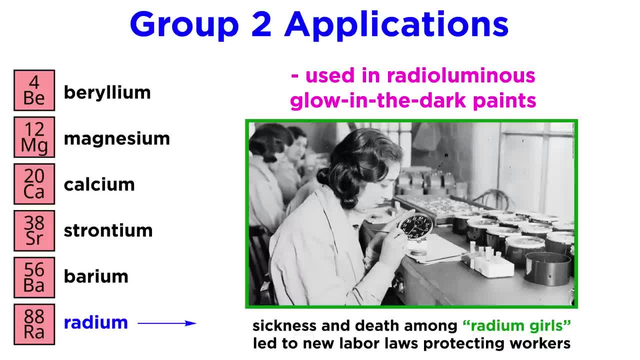 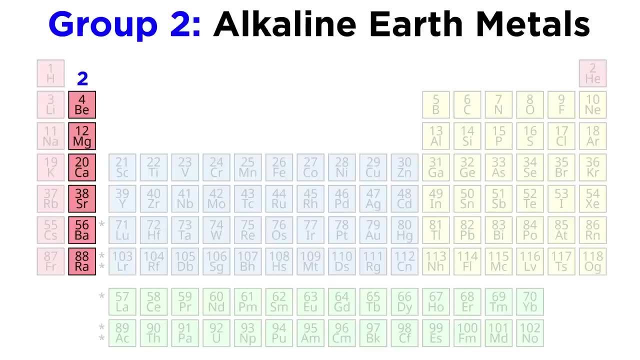 causing them to ingest enough radium to lead to many cases of sickness and death. This brought about new labor laws protecting workers from undisclosed dangers, And with that we complete a summary of the alkaline earth metals which represent group two on the periodic table. Subtitles by the Amaraorg community.